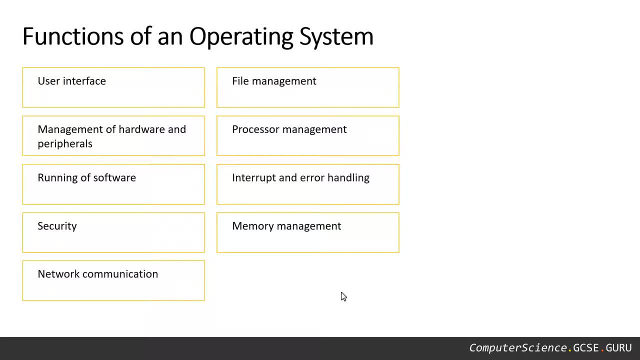 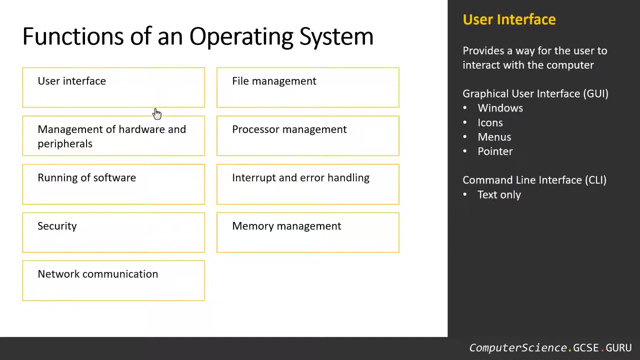 functions in a bit more detail. We have the user interface. we have file management, the management of hardware and peripherals, processor management, the running of software, interrupt and error handling, security, memory management and network communications. So let's take a look at the user interface. 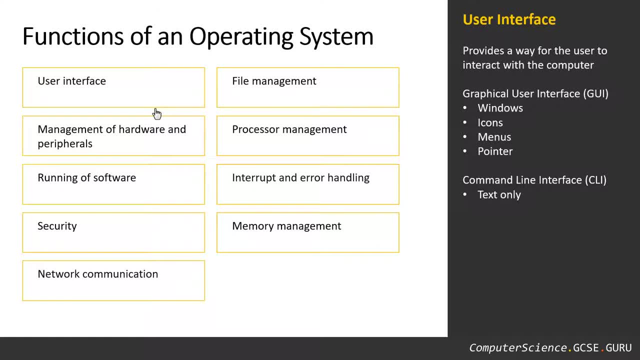 So the operating system provides a way for the user to interact with the computer. Historically this was done with a command line interface which used just text only. but most modern computers now will use a graphical user interface or a GUI to allow us to interact with the computer. A GUI has windows, icons, menus, pointers as a way of interacting. 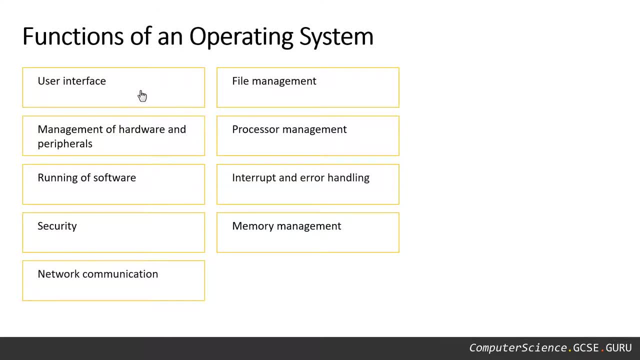 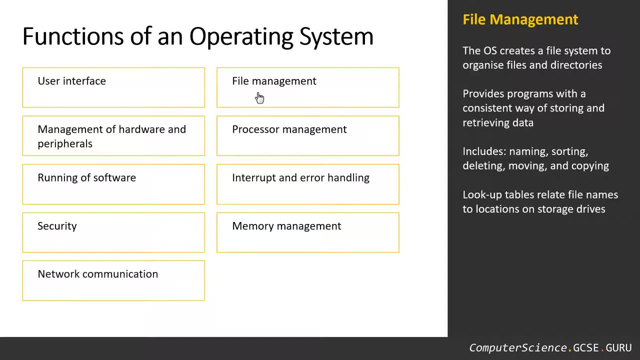 Another feature of an operating system is the management of files. The operating system creates a file system that organizes files into directories on the computer. These names are going to a lookup table and the locations are remembered. It provides programs with a consistent way of storing and retrieving data from storage. 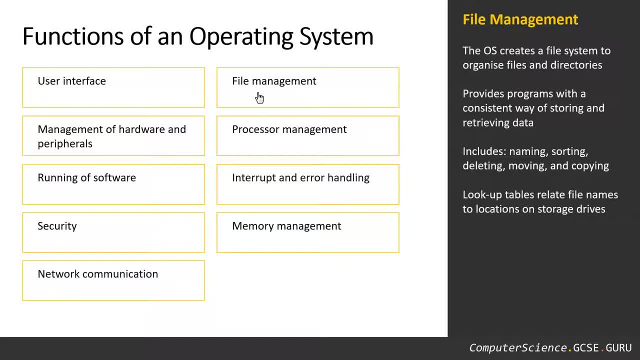 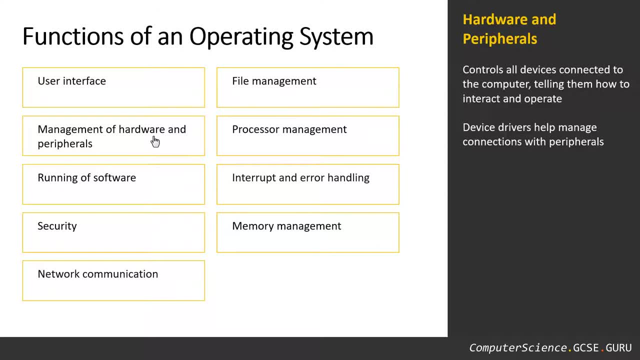 So the operating system controls all devices that are connected to the computer and it tells them how they are to interact and to operate. Peripherals can include a hard drive, portable storage, USB ports and so on. Each peripheral, so each device you connect to a computer, will have its own rules. that 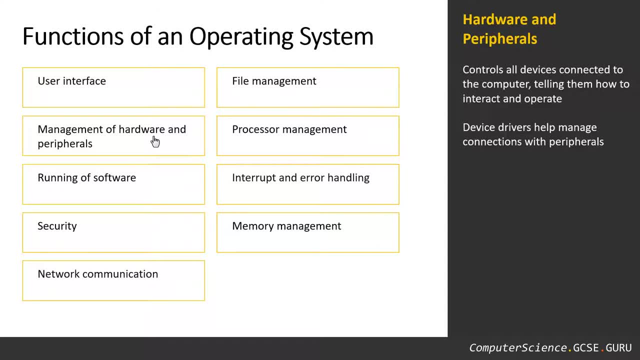 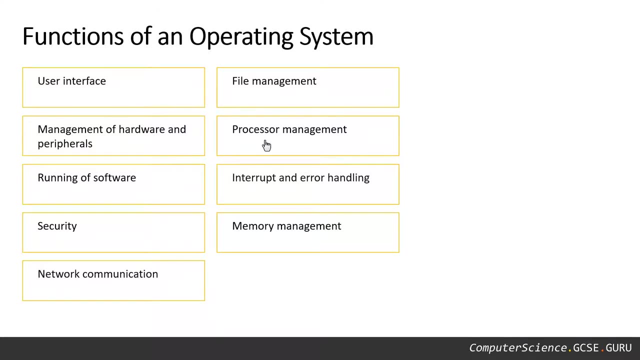 dictate how it can transmit data to the computer. In order to not get confused, the operating system will use something called device drivers to learn how to use those peripherals and to allow communications to take place effectively. Okay, next up, we've got the management of hardware. 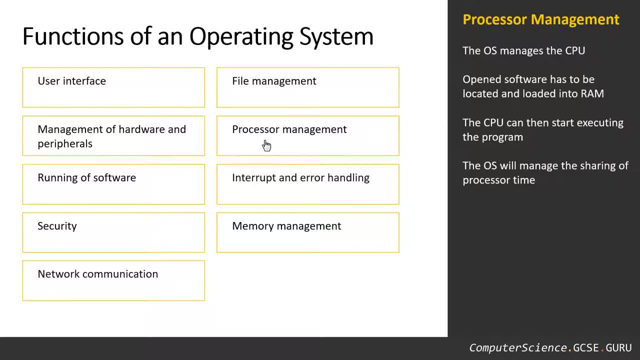 Next feature of an operating system is processor management. The processor, the brains of the computer, needs someone or something to manage it. The operating system will manage the processor. When a program gets opened, the operating system will find it on the hard drive and 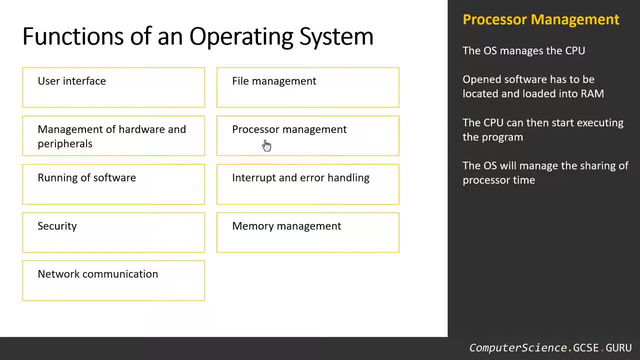 load the instructions into RAM, into the temporary memory. It will then tell the CPU, the processor, that it can start to execute that program. The operating system will then tell the CPU, the processor, that it can start to execute that program. 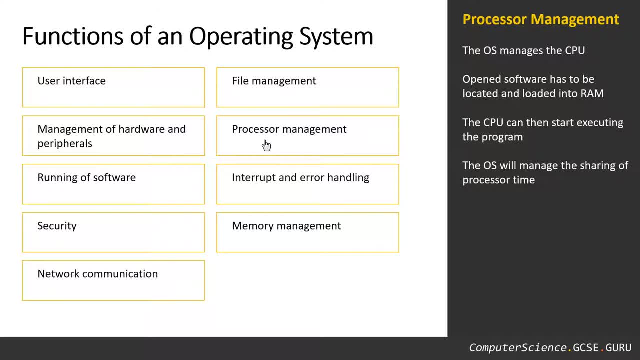 The operating system will also manage the sharing of processor time. If there's more than one program that needs time with the processor, it's down to the operating system to prioritize and to manage that time appropriately. Okay, running of software. We all really know that to run software we need an operating system installed first. 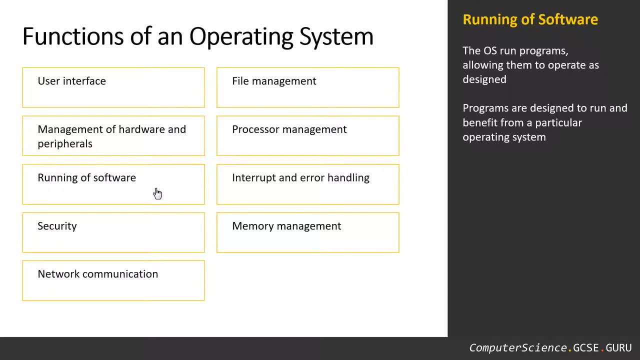 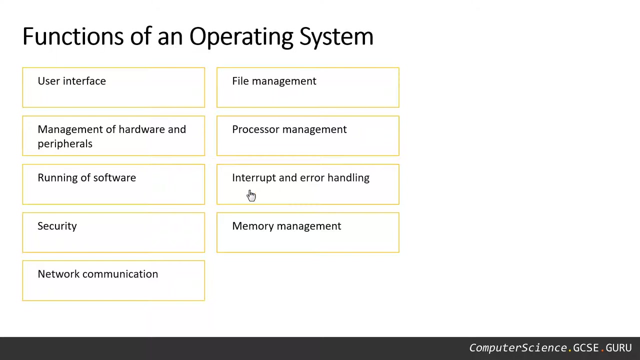 and then the software is installed on top of the operating system. Doing this allows programs to benefit from the features of an operating system, such as the existing communications and connected hardware and file management systems. without the operating system, you wouldn't be able to install programs to work okay. leading on. 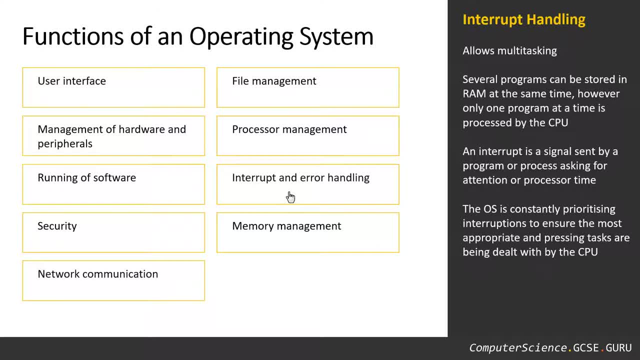 from processor management. we have something called interrupt handling. now we know that several programs can be stored in RAM at the same time, but only one at a time can be processed by the CPU. in order to give the illusion of multitasking, we use interrupt signals. so each task, each program is fighting for. 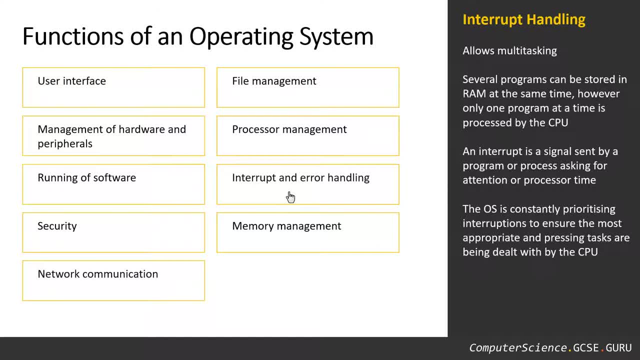 attention and it's up to the operating system to prioritize those interruptions and to give the most important task, the most pressing tasks, to the processor to complete, while the rest go into a queue. so the operating system is constantly prioritizing interruptions to ensure the most appropriate and pressing tasks. 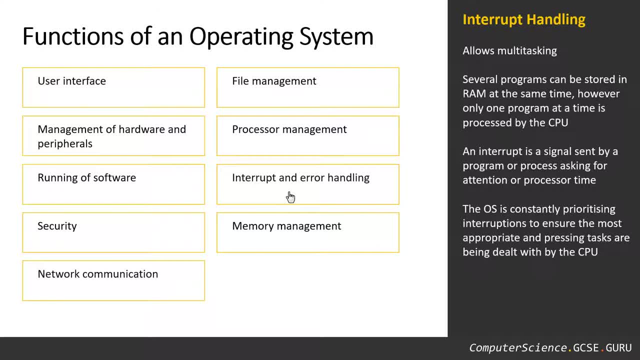 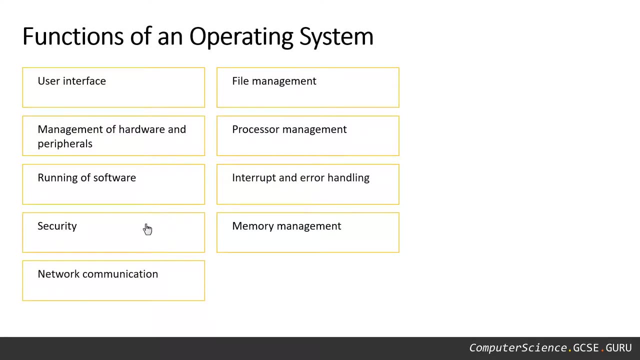 are dealt with by the CPU, but because this happens hundreds or thousands of times a second, we don't notice this. we just feel as if all these programs are all working together at the same time, but in fact they're not. it's a constant juggling act. 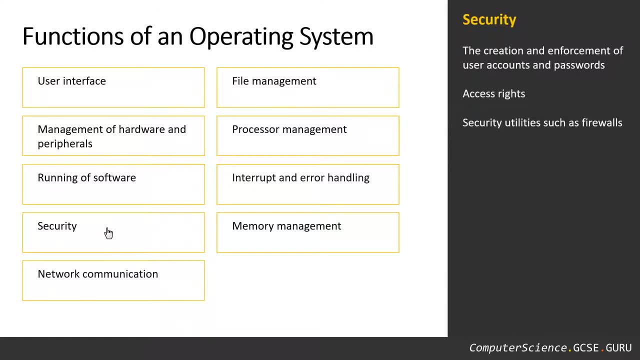 security. so an operating system has an important role to play in the security of your computer as well. if you've got several people using the same computer, then the operating system will allow you to create separate user accounts and passwords, and it's the operating system that enforces those rights to ensure you.